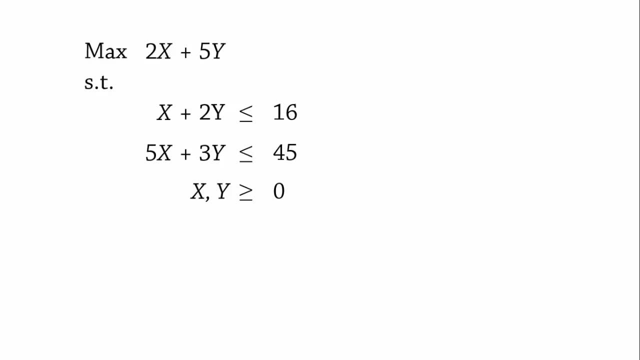 to buy, produce, sell or transport and so on. The 2x plus 5y here is referred to as the objective function which we want to maximize. In linear programming we either maximize or minimize the objective. The next two lines are called constraints. They are restrictions, that 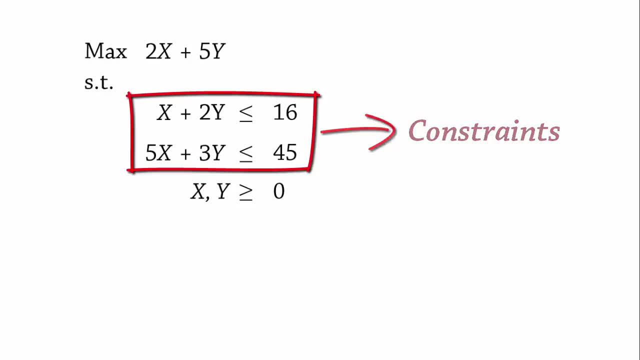 shape how you attain the objective. Let's call them C1 and C2 for reference purposes. Since we're dealing with real-life objects, we're going to use the C1 and C2 for reference purposes, Since we're dealing with real-life objects. 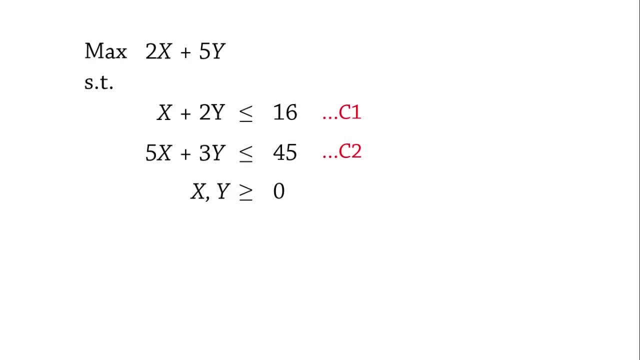 we do not expect them to have negative values. So the last line here tells us that both x and y have to be greater or equal to zero. We call them the non-negativity constraints. To solve the model graphically, we begin by finding points that satisfy the constraint lines. 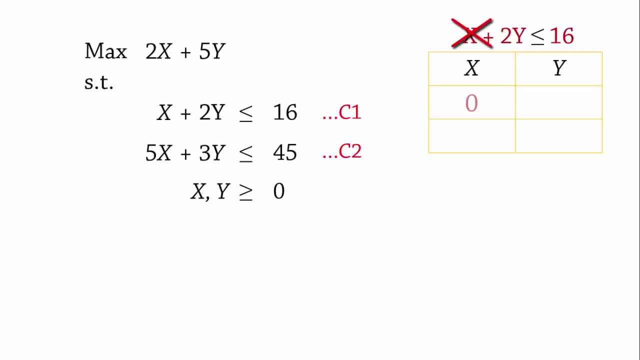 For the first constraints: when x equals 0, y equals 8. And when y equals 0,, x equals 16.. For second constraint: when x equals 0, y equals 15, and when y equals 0,, x equals 9.. 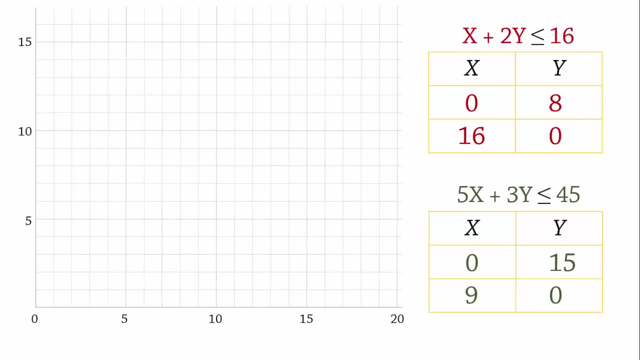 Now, when drawing the graph, we usually just stay in the first quadrant here, where both x and y are positive, because of the non-negativity constraints. So for the first constraint we have the points and We join those two points for the constraint line. 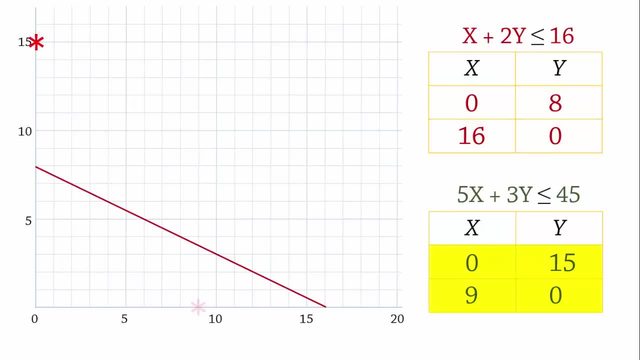 We do the same for constraint 2, and then draw the constraint line. Since these constraints are less than or equal to constraints, they will be satisfied in the region below the lines towards the origin. Therefore, the region satisfying both constraints simultaneously is this one here. 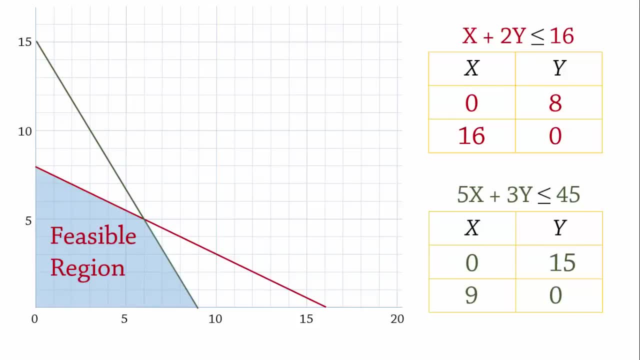 It is called the feasible region. That is, any point in this region is a feasible solution. In particular, the optimal or best solution is the feasible solution. The best solution will occur at an extreme point or corner point of the feasible region. These are the corner points for the feasible region. 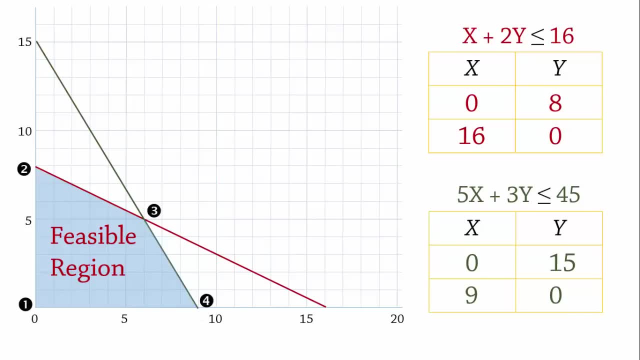 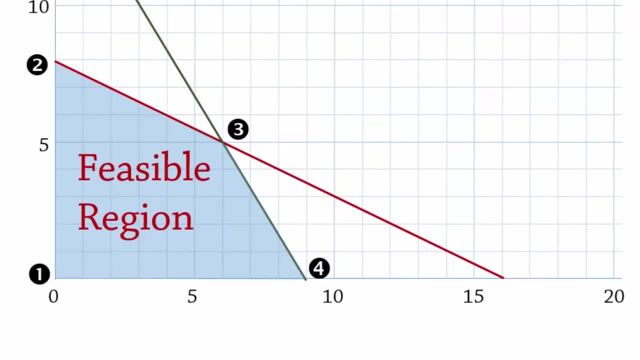 Let's label them 1 to 4.. The optimal solution to this linear programming problem will occur in at least one of them. To decide which one is optimal, we will find the coordinates of the points, plug them into the objective function and then choose the best. 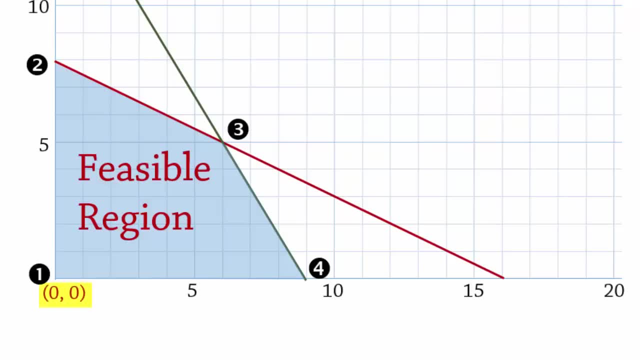 At corner point 1, the coordinates are clearly visible, Clearly: 0, 0.. At point 2, 0, 8.. At point 4, 9, 0.. Now, those are easy to see. For corner point 3, we can see that the coordinates are 6 and 5 by eyeballing. 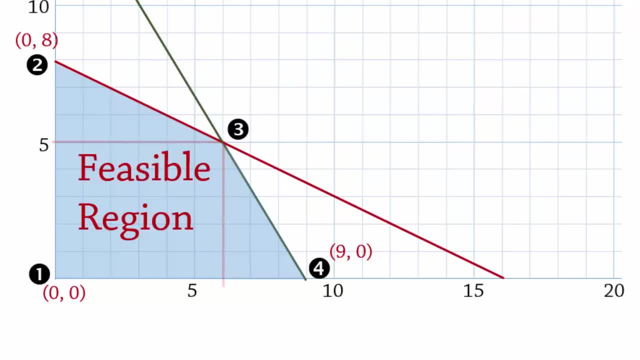 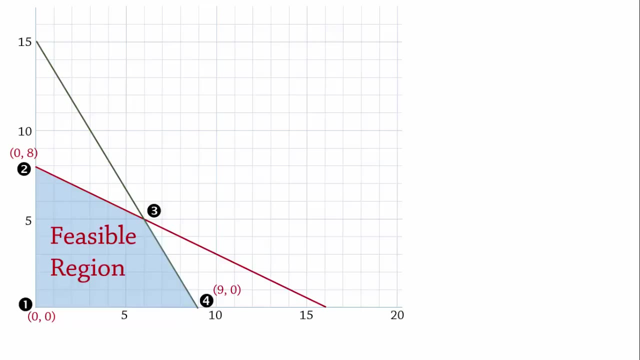 That is looking at it very closely. But eyeballing is not usually the best way to go when finding the intersection of two lines, Especially when manually drawing the graph. So let's see a way to solve the two equations simultaneously. Here are the lines for the two constraints: 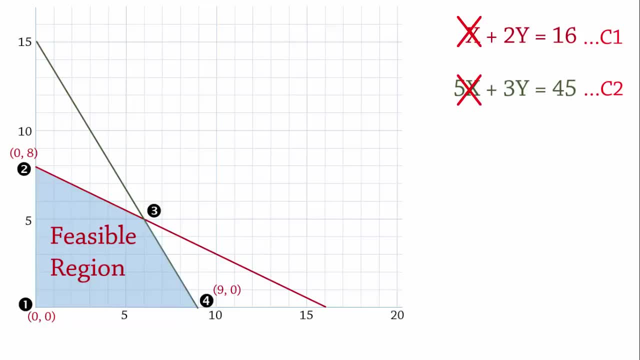 Now suppose I choose to eliminate x. Note that the coefficient of x here in C2 is 5.. Then I can simply multiply the first equation by 5. to give 5x plus 10y equals 80. And then we can subtract C2 from the new equation. 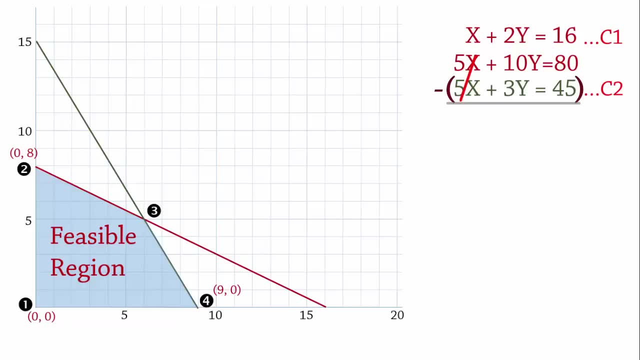 So 5x cancels 5x, 10y minus 3y is 7y, And 80 minus 45 gives 35. And on dividing both sides by 7, we have y equals 5.. To now find x, we substitute y equals 5 into any of these three equations. 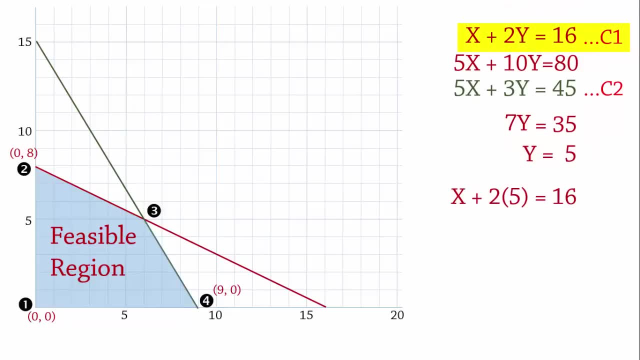 Suppose we choose C1. Then we have x plus 2 times 5 equals 16. That is, x plus 10 equals 16. x equals 16 minus 10. And x equals 6. So the x- y coordinates for extreme points are the same. 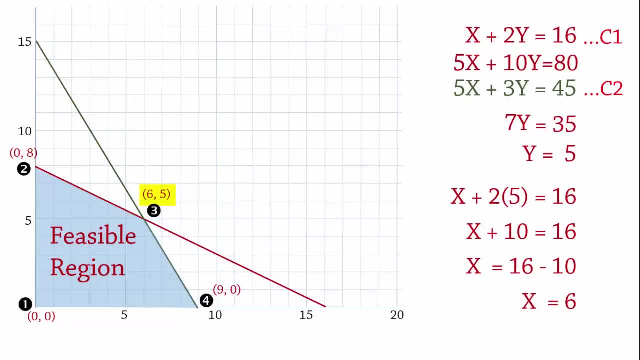 So the x- y coordinates for extreme points are the same, So the x- y coordinates for extreme points are the same, And 3 are indeed 6 and 5.. Next we determine the optimal solution point by finding the corner point that gives the 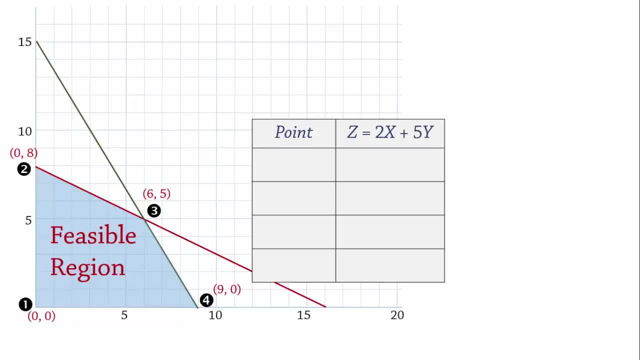 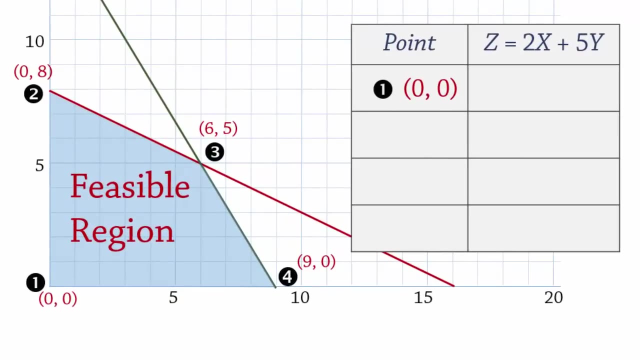 best value of the objective function. The objective function was to maximize 2x plus 5y. As you can see here the objective function or its value is sometimes represented with z. So now the x- y coordinates at point 1 are 0,, 0, and substituting that in the objective